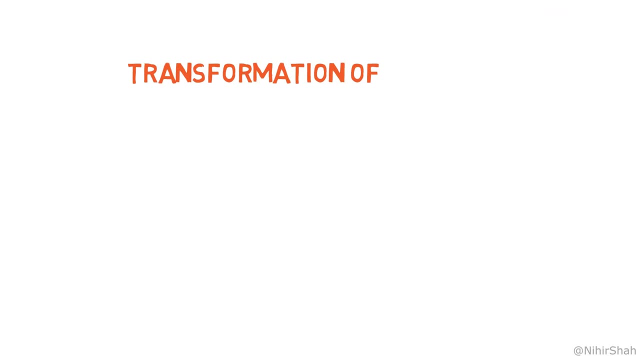 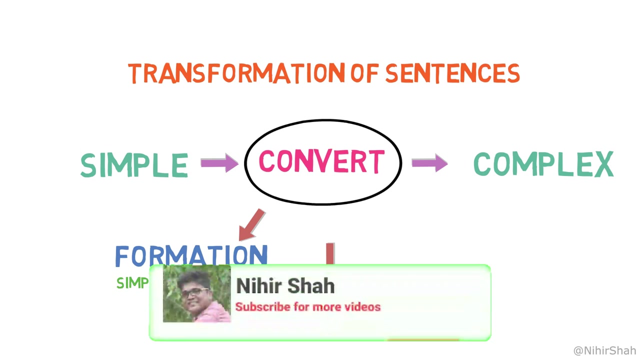 Hello friends, welcome to the series on transformation of sentences. In this video, we will learn how to convert a simple sentence into a complex sentence. First we will learn how a simple sentence is formed and how a complex sentence is formed. Then we will look into the steps to convert a simple sentence into a complex sentence. 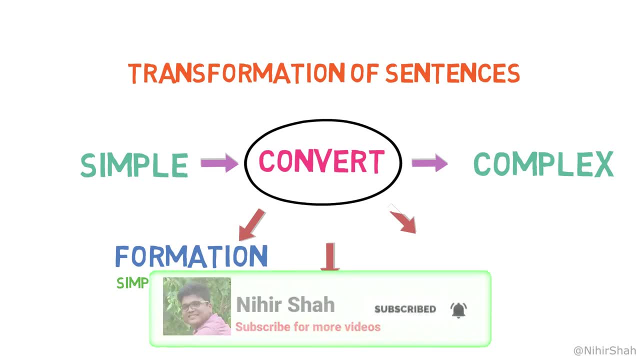 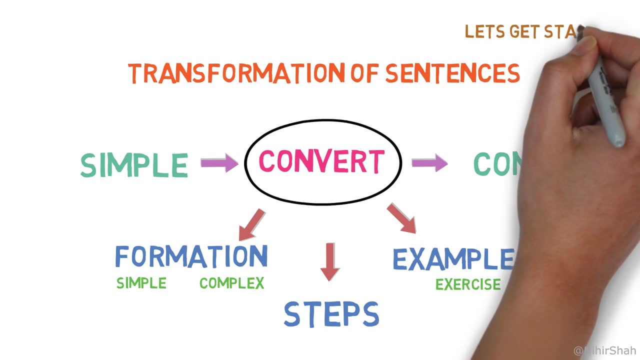 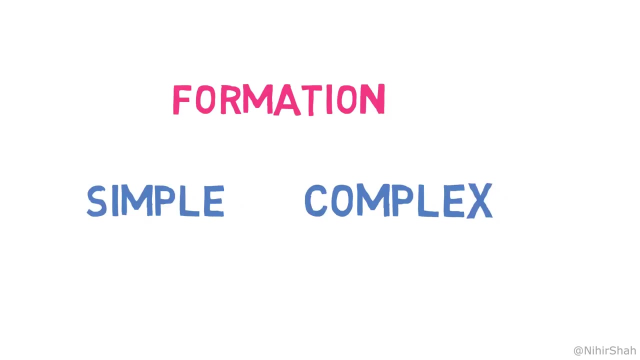 without changing the meaning of the sentence. Finally, we will understand it with examples and I will give you an exercise to practice. So, without further ado, let's get started. Let's first learn the formation of simple and complex sentences. What is a simple sentence made of? 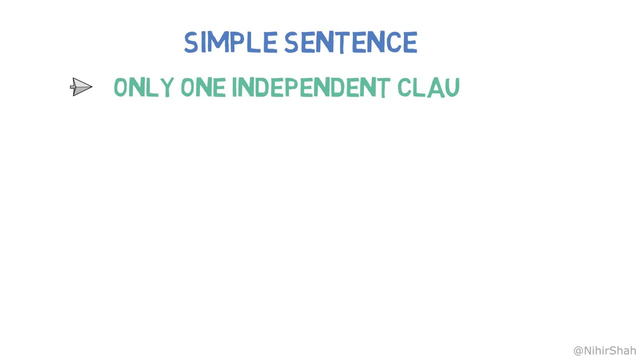 A simple sentence has only one independent clause. This means it has only one subject and one predicate, and it will have a complete meaning by itself. However, it may contain only one idea or thought, or more than one idea or thought. For example, he is very weak. 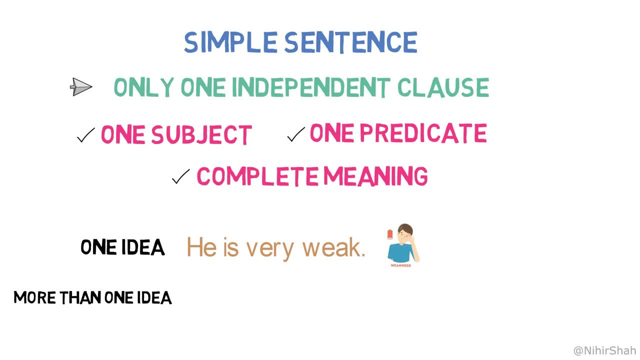 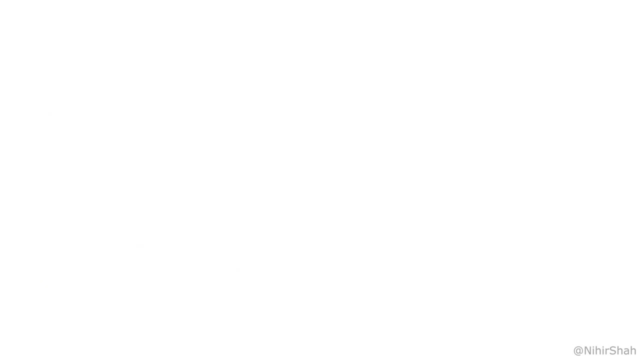 Here there is only one idea. However, look into this sentence: He is too weak to run fast. Here there are two ideas. One is he is very weak and the second is to run fast, which is linked to the first idea. Now let's learn what is a complex sentence made of. 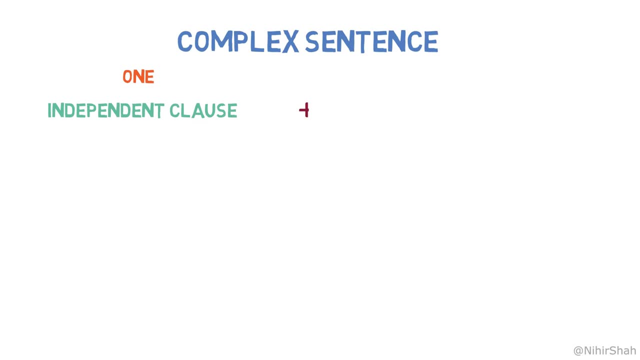 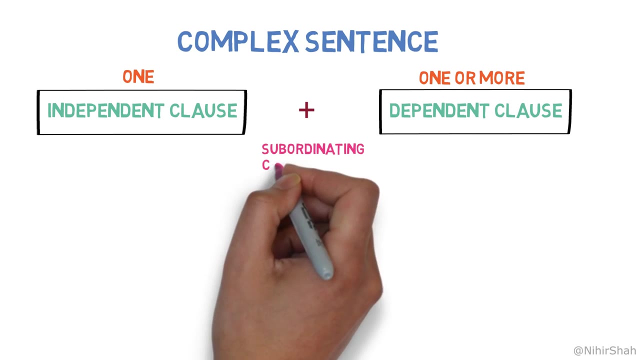 It is made of one independent clause and one or more dependent clause. The independent and dependent clauses are joined with a subordinating conjunction. Let me write this sentence that he cannot run fast Here. this sentence is having a subject- he and verb run- and it is also having a meaning. 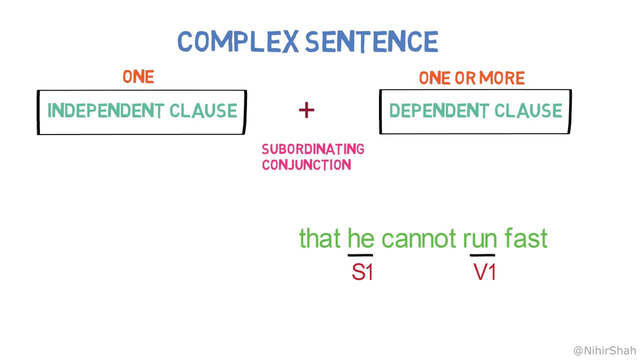 However, we feel that the complete sense or meaning is not there, So it's a dependent clause. It is made of one independent clause and one or more dependent clause. Now look at this sentence. He is so weak. Here he is the subject and is is the verb. 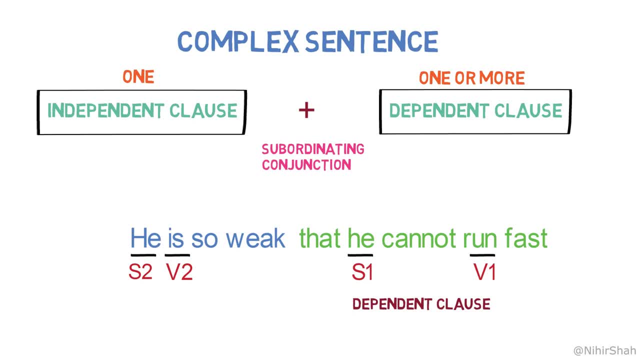 This sentence is giving a complete meaning by itself, So it's called an independent clause. Now let's combine these two clauses and the final sentence is: he is so weak that he cannot run fast. Here there is one independent clause and one dependent clause. 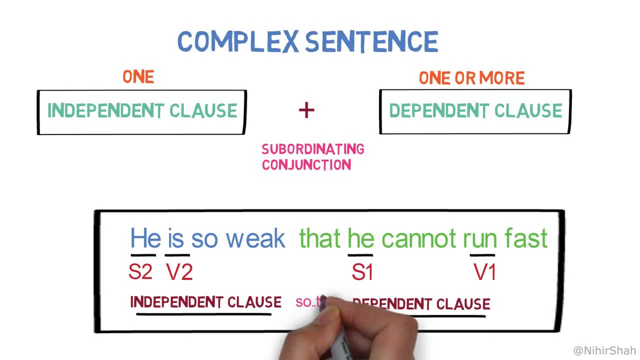 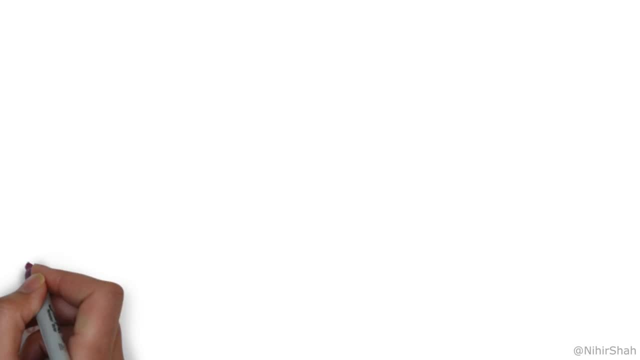 And it is joined by subordinating conjunction so that So to form a complex sentence, you would require an appropriate subordinating conjunctions. You might be wondering what are all the subordinating conjunctions that you must remember, So let me share with you all the most important subordinating conjunctions. 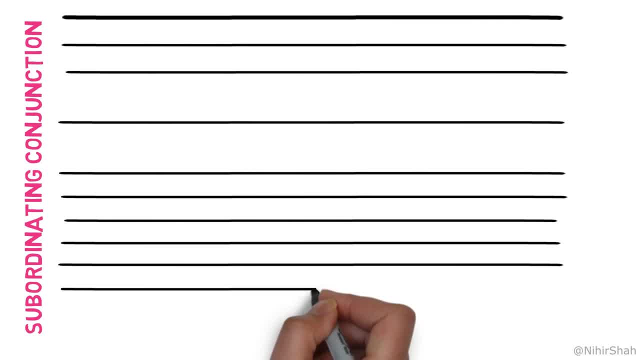 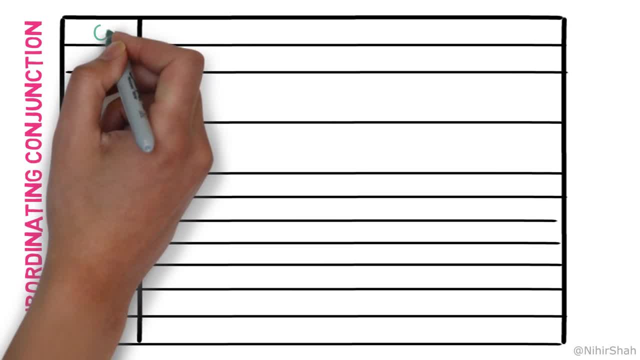 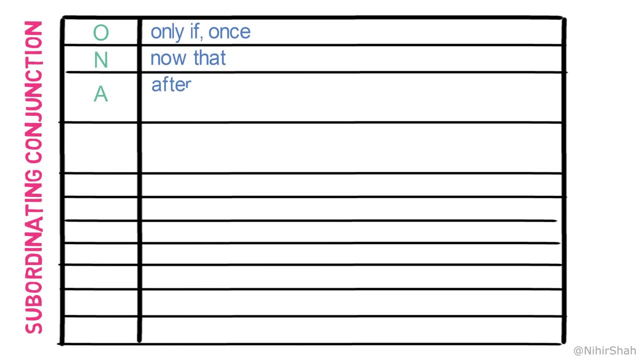 I will list down the first letter of each conjunction in the left hand side and all the related conjunctions in the right hand side of the table. Oh, only if, once and now, that a after although as as long as, as much, as, as soon. 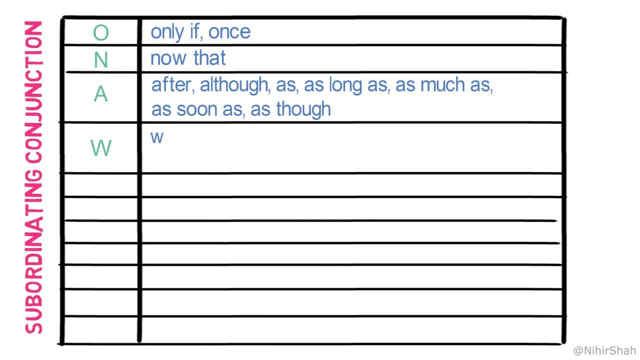 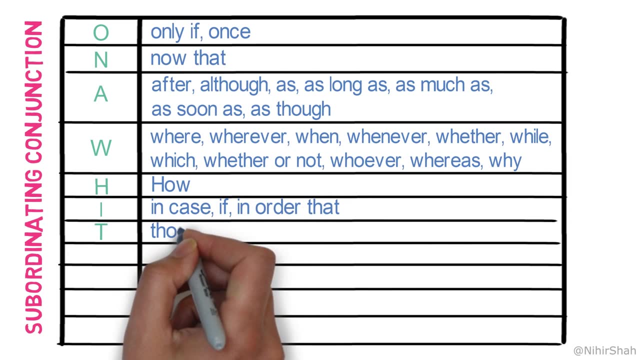 as as though w, where, wherever, when, whenever, whether, while, which, whether or not, whoever, whereas, why a? How, I, In case? if in order that t Though, then that 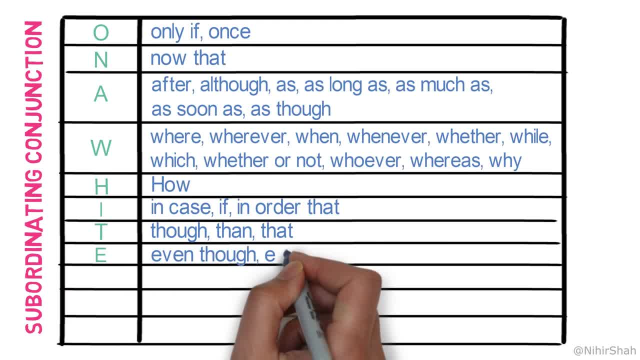 e Even though, even if b Before, because u Until unless s Since, so that. So this is the list of conjunctions. There are two subordinating conjunctions. There are too many conjunctions. 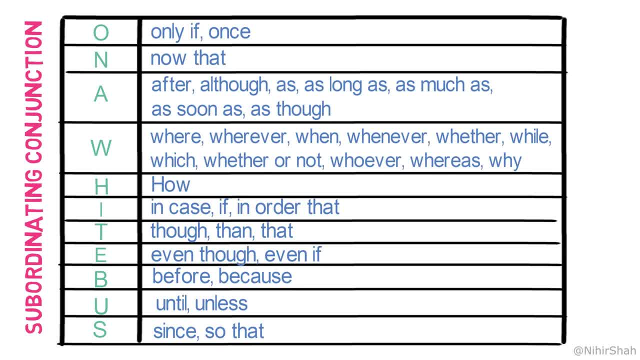 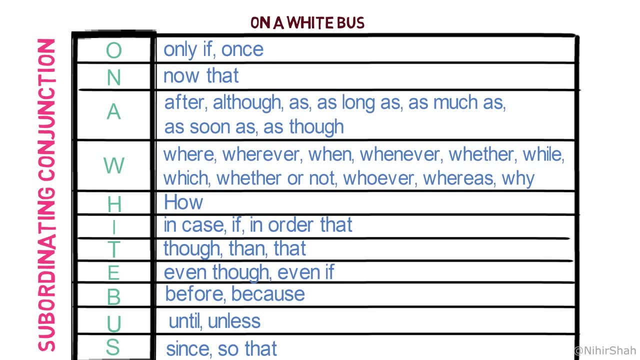 But let me give you a trick to remember all of them. I have just picked the first letter of all of them and made this phrase on a white bus. So just remember this phrase on a white bus and you will surely remember all the conjunctions. 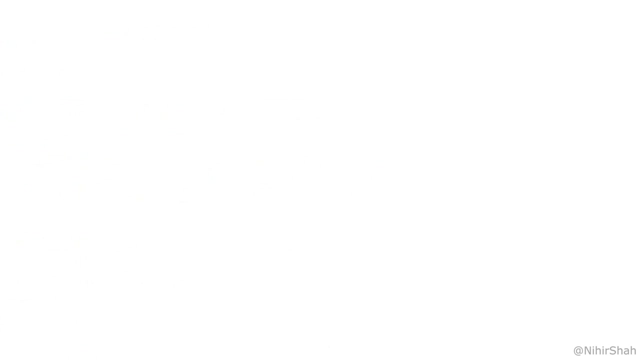 if you do a lot of practice. Now, if you remember, we looked into this example of the simple sentence: He is too weak to run fast. weak to run fast. and for the complex sentence, the example was: he is so weak that he cannot run fast. 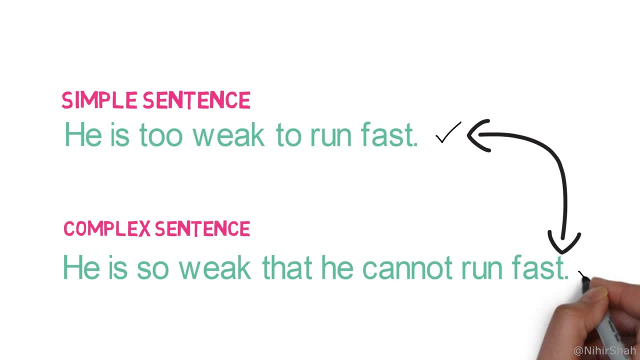 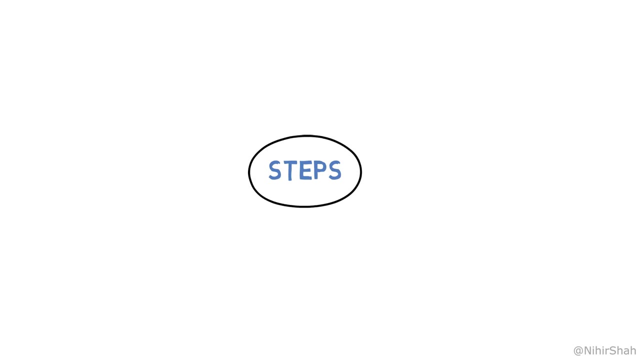 if you notice closely, the meaning of both the sentences is identical. this is called the transformation of a simple sentence into a complex sentence, without changing the meaning. now let's learn the three step formula to convert a simple sentence into a complex sentence. the steps are: number one: identify the main idea and other ideas given in the simple sentence. number two: convert. 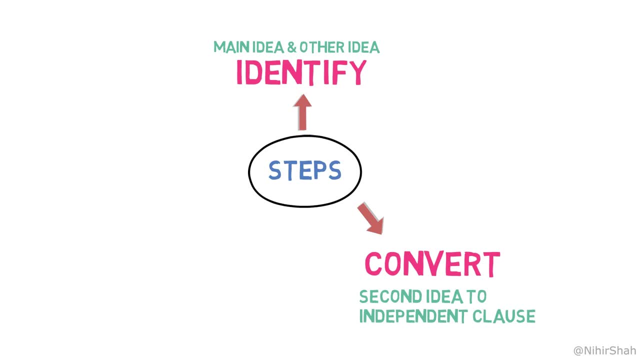 the second idea into an independent clause. and number three, add appropriate subordinating conjunction to the clause to make it a dependent clause and form the sentence with some of the changes if required. the simple way to understand the steps is that you need to expand a word. 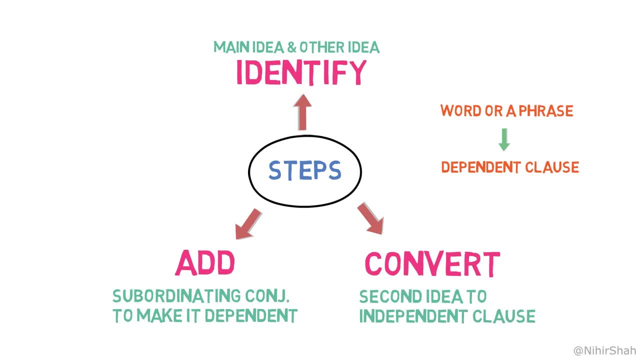 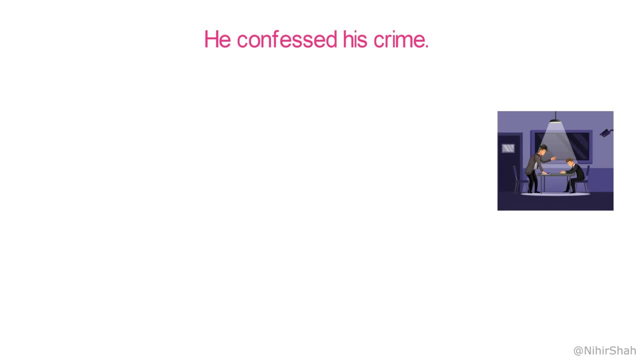 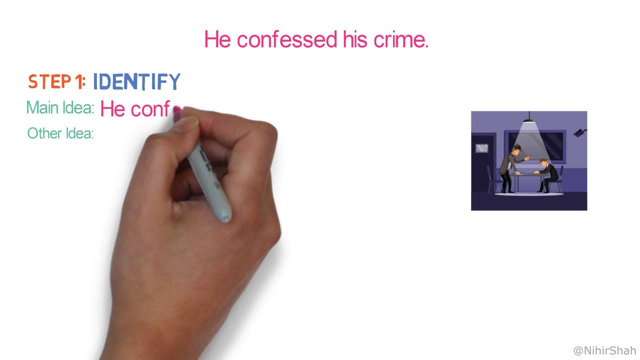 or a phrase into a dependent clause. so this is the three step formula. let's understand it with an example. he confessed his crime. step one: identify the main idea and other ideas given in the simple sentence. here he confessed is the main idea and his crime is the second idea. step two: convert the second. 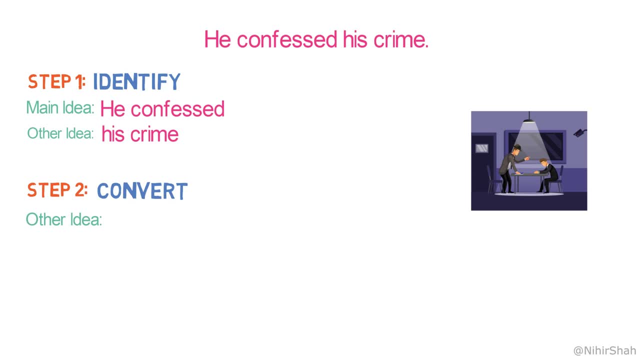 idea into an independent clause. here we have converted the phrase his crime to a clause he is criminal. and step three, it is to add the most appropriate subordinating conjunction. so here i have used that as the conjunction. so the final sentence is: he confessed that he is a criminal. observe these steps carefully. let's look into next example. 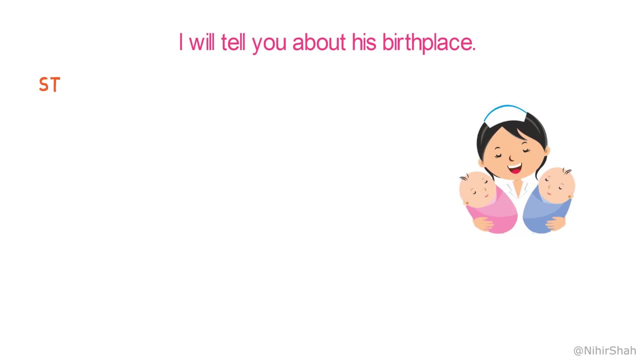 i will tell you about his birthplace. step one: here the main idea is i will tell you, and the secondary idea is his birthplace. step two: we are converting the secondary thought- his birthplace- into an independent clause: he was born. step three: we are using the conjunction where here, so the final. 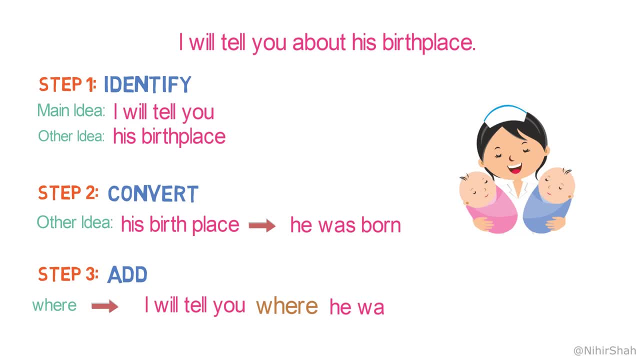 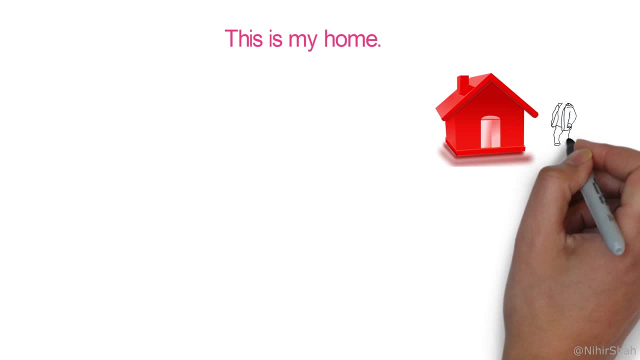 sentence is: i will tell you where he was born. let's look into next example. this is my home. now. this is an interesting sentence. it seems that there is only one idea and won't be able to convert it into a complex sentence. However, when you break it, you will get some more clarity. 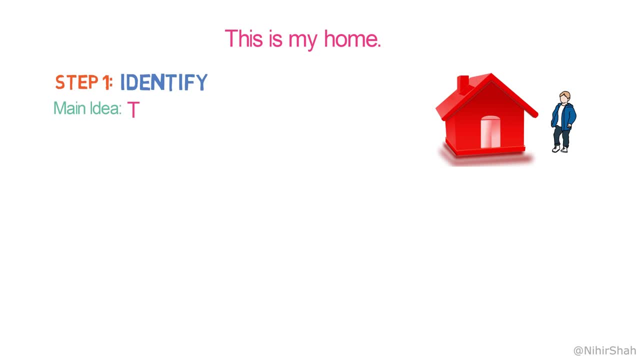 Let's try it. Step 1.. The main idea is: this is a home And the secondary idea is: this is my home. Step 2 is to form an independent clause using the second idea. Here we can ask ourself: what is the use of home? we live there, right? 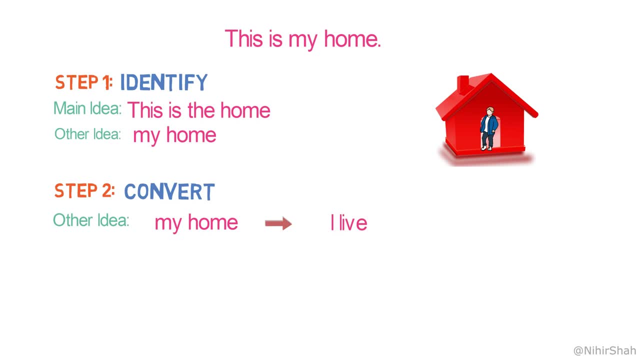 So we can write the second clause as I live, So we have now an independent clause. Step 3 is to join them with an appropriate conjunction. Here I have used where, So the final sentence is: this is the home where I live. 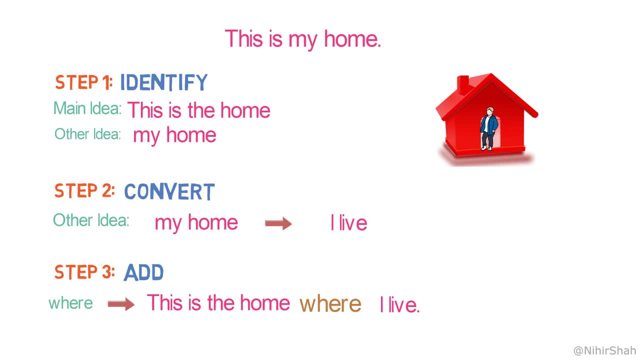 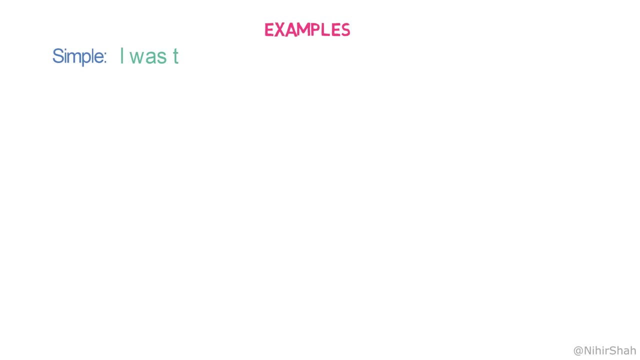 I hope now you are clear on the steps. I would be giving you some more examples without explaining the steps in detail. Simple sentence: I was the first To hear the news Converting it into a complex sentence it becomes. I was the first who heard the news. 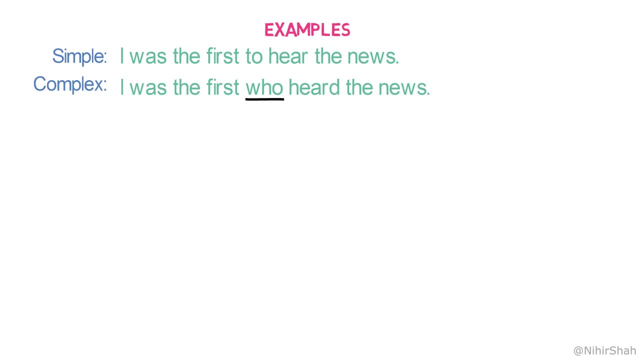 Please note here who is also acting as a subject of the dependent clause. Let's look into next example. Being quite contented, he never complained. Converting it into a complex sentence it becomes: Since he was quite contented, he. 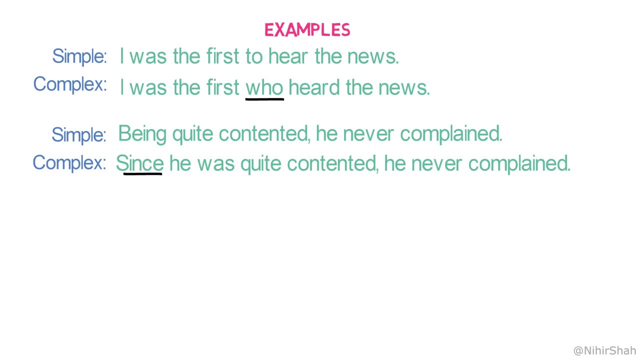 never complained Here, since is the subordinating conjunction With your name. With your permission, I will go away, Converting it into a complex sentence. it becomes: If you permit, I will go away In spite of the heat. they marched quickly. 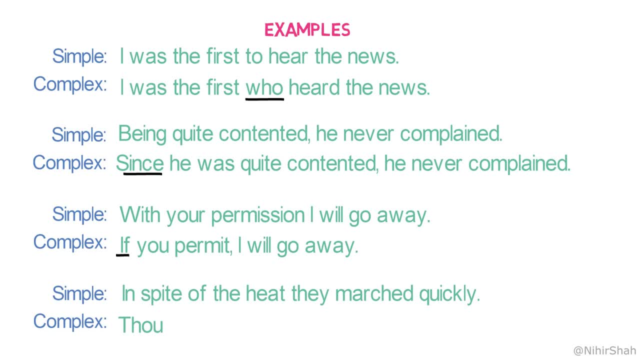 Converting it into a complex sentence, it becomes- Though it was hot, they marched quickly. Here, though, is the subordinating conjunction. I hope now you will be able to convert a simple sentence into- I was the first- A complex sentence. 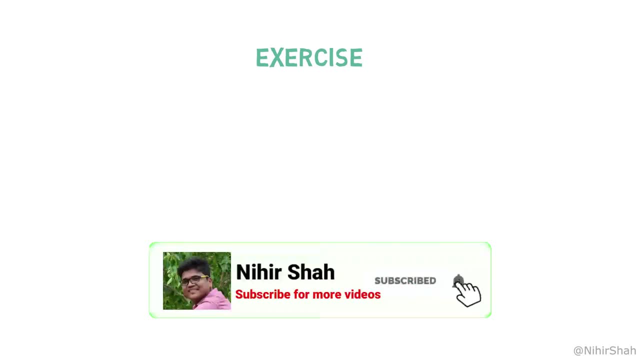 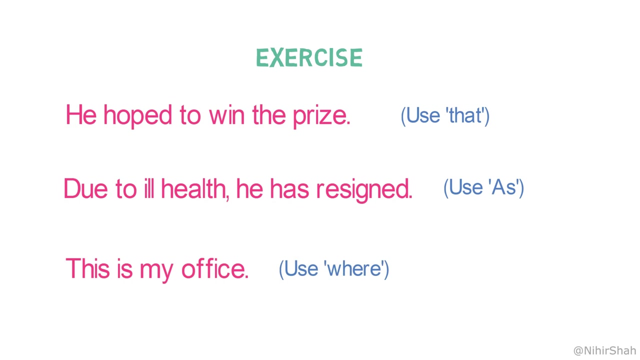 Now let me give you an exercise to practice. Here. you need to convert a simple sentence to complex The sentences: are He hoped to win the prize? Due to his ill health, he has resigned. This is my office. Hints are also given to solve these questions. 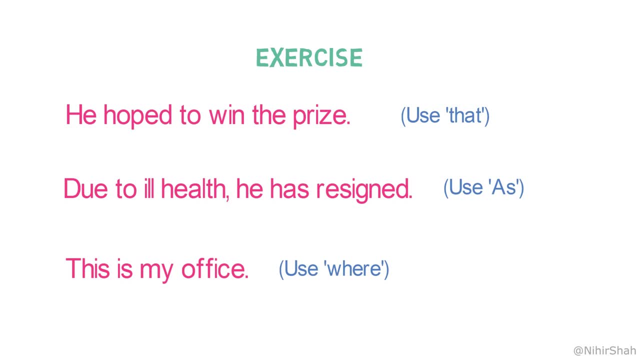 Pause the video, Solve and message the answers in the comments. For correct answers, please check the description of context from the end of the video. Thanks for watching this video. Please subscribe to this channel. By doing so, you can ask any questions.